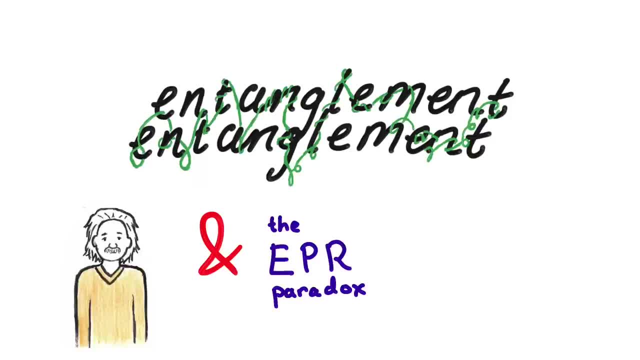 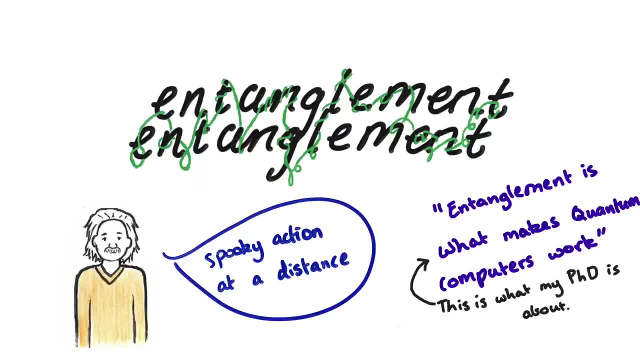 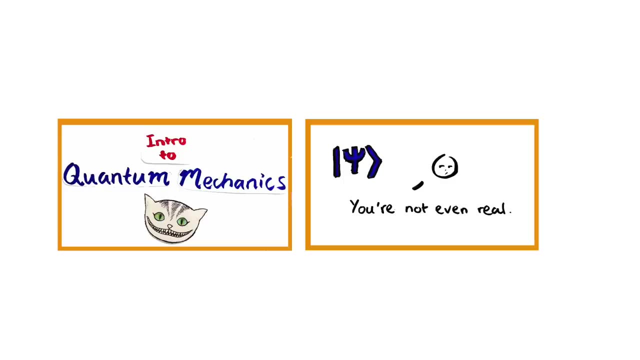 Entanglement is often blamed for all the spooky weirdness of quantum mechanics. In this video I'll explain what it really is and one of the coolest consequences: the EPR paradox. If you haven't watched any of my other videos on quantum mechanics, you might want to watch. 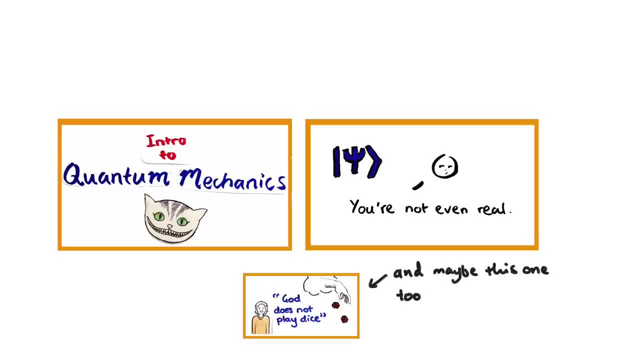 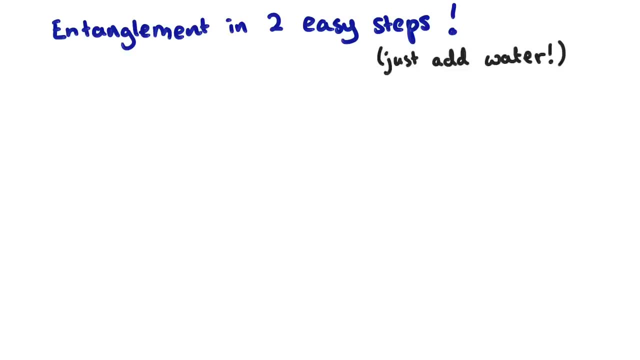 these two, but I'll have a really quick recap for everyone's benefit. There are only two quantum rules that we need to give us entanglement. The first is the superposition rule. It says that if there are several options for an object and there's 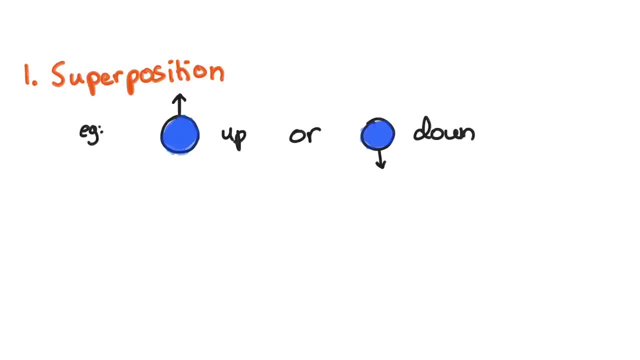 no way that anything could know what option the object is really doing, then it is in a superposition of doing all of them. Now, importantly, this is very different from saying it is doing one or the other but we don't know which. For example, if you flipped a, 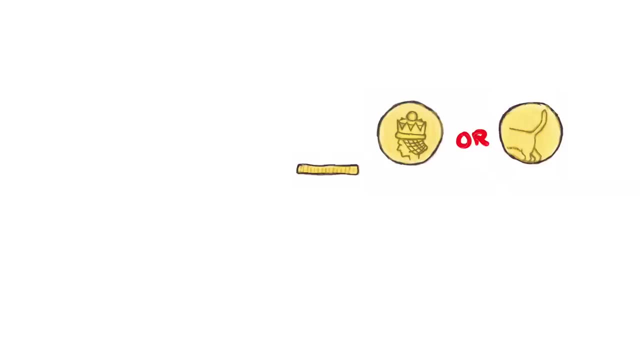 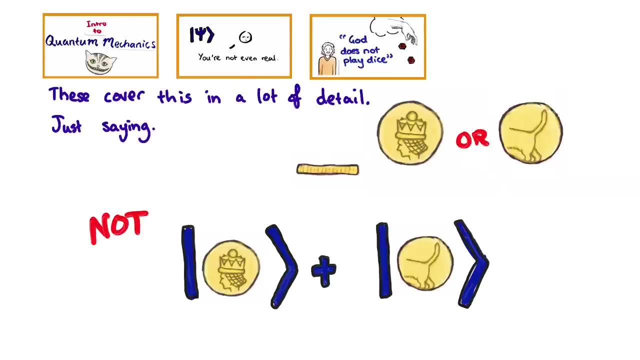 coin. you may not know whether it's heads or tails, but this doesn't mean it's in a superposition. You know the coin is one or the other, But you're not sure which. A superposition is a state where a particle seems to really. 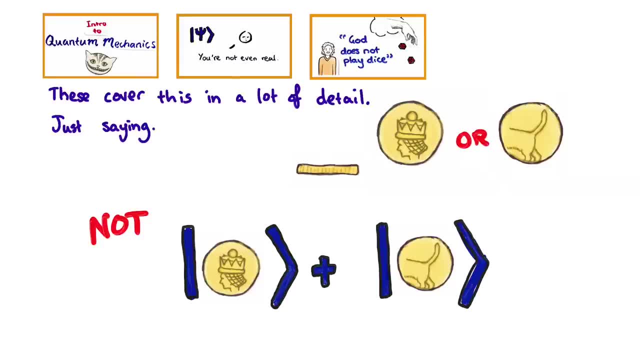 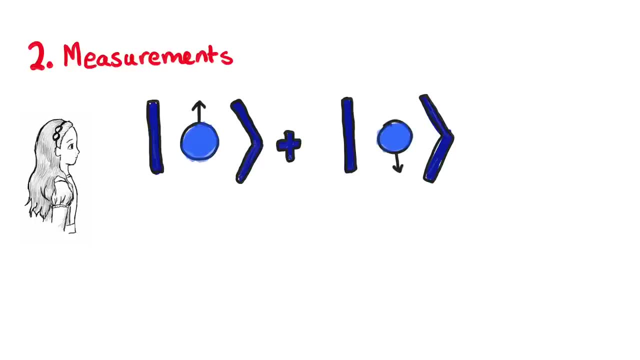 be doing both at the same time, at least in some interpretations of quantum mechanics. Then there's the measurement rule, that if you measure a particle that's in a superposition, it must collapse to just one of the options in its superposition. 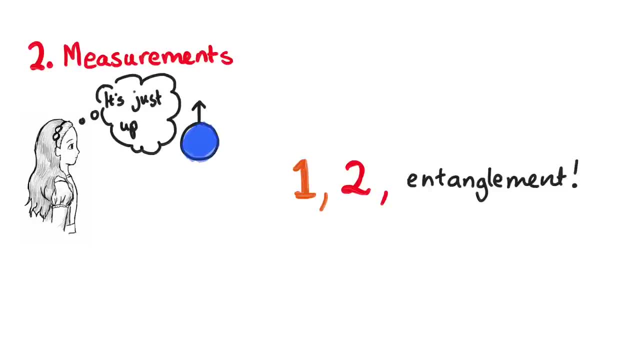 Here's how all of this can naturally lead to entanglement. We'll take an example using spin, but if you don't know what that is, don't worry too much. Imagine we have a very energetic particle of light. Then, using Einstein's famous formula, 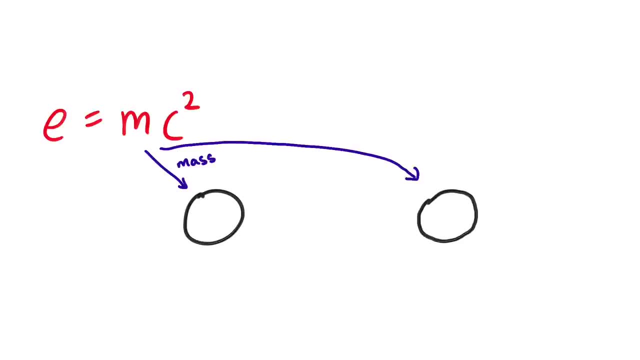 it can convert that energy into mass. For example, it could form two new particles, But there are a bunch of conservation laws in physics that restrict what these particles are and what they do. For example, a photon has no electrical charge, so these new particles 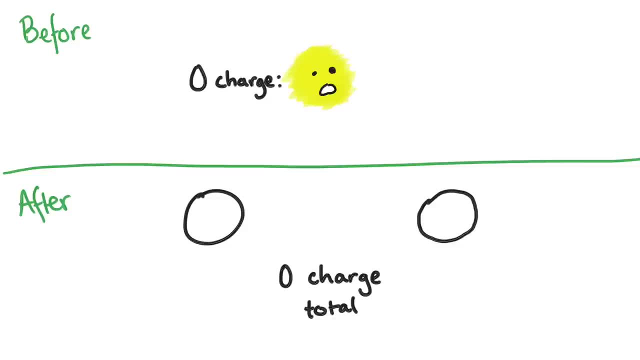 should have no net charge. So one could be an electron, but then the other has to be a positive version of an electron, a positron, so that in total their charge is zero. But there's also a thing called conservation of spin. Photons never have any spin, but 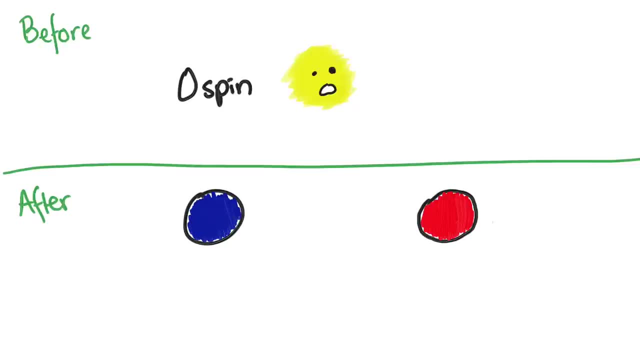 both electrons and positrons do. They can either have spin up which is positive, or spin down which is negative. So for their total spin to cancel, one should be up and the other down. But which way is which? Usually you'd want to say it's one of these ways, but you don't. 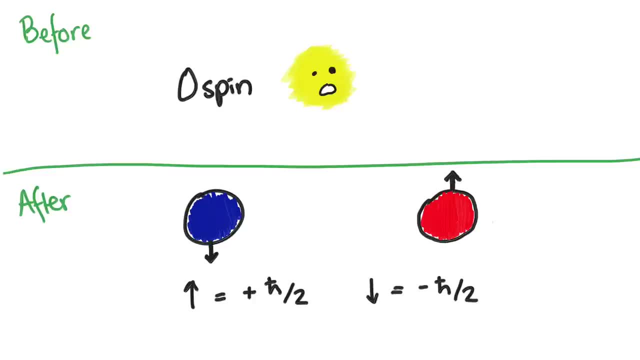 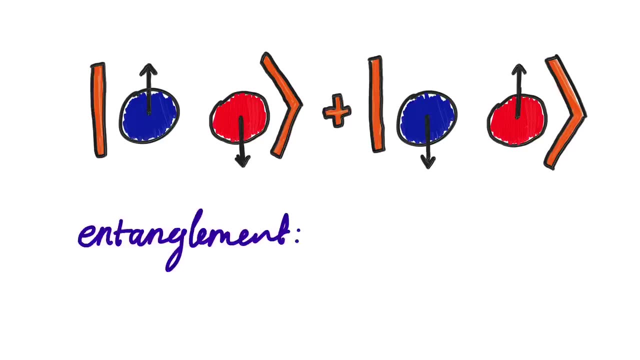 know which. However, remember, in quantum mechanics, if there is no way to know, then it must be a superposition of both. This state is entangled, but you may not see what's so special about it yet. Entanglement is the crazy property that it's impossible to describe the state of one of these particles. 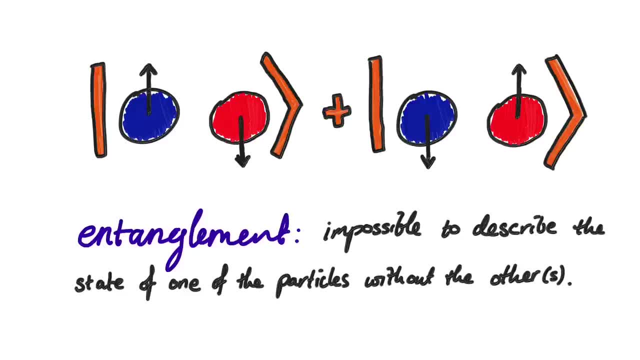 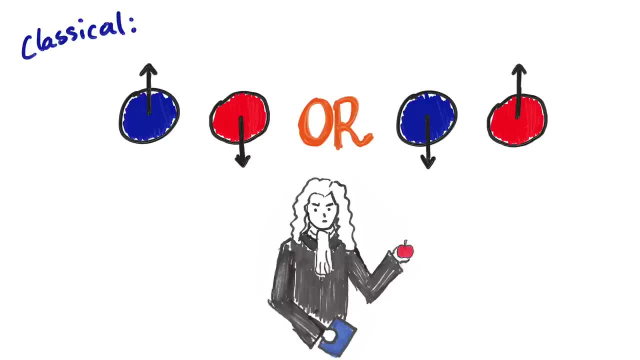 without mentioning the other. To see what this means and why it's unique to quantum mechanics, let's compare it to the not-quantum scenario. So classically we'd think it has to be one or the other of these cases, but not both. it's just that we don't. 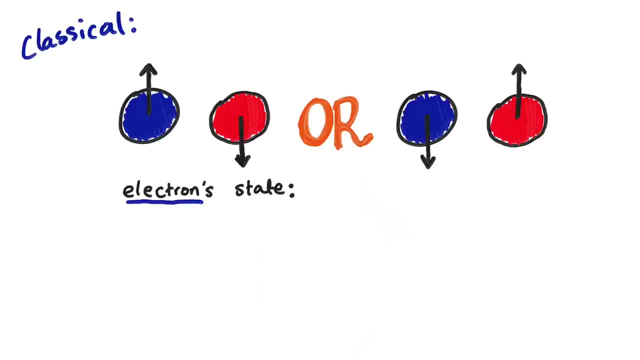 know which Here. if I wanted to describe the state of the electron, it would be up if the positron is down and down if the positron is up. This seems like it fits my definition of entanglement – it's impossible to describe the state of the electron without 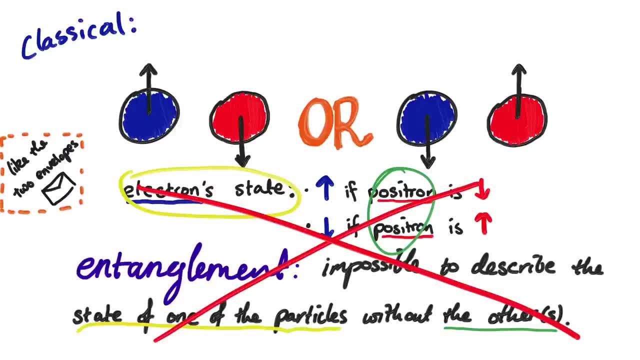 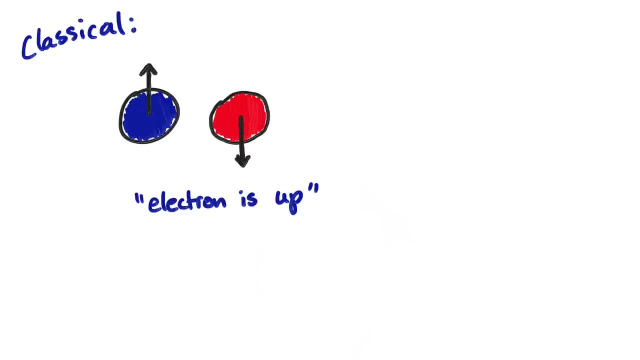 talking about the positron. So why is it so important to know which is which? Why is it so important to know which isn't this entanglement? Because really, the particles are just doing one thing. let's say this one. If I knew that, then I could say: the electron is up. It's only because 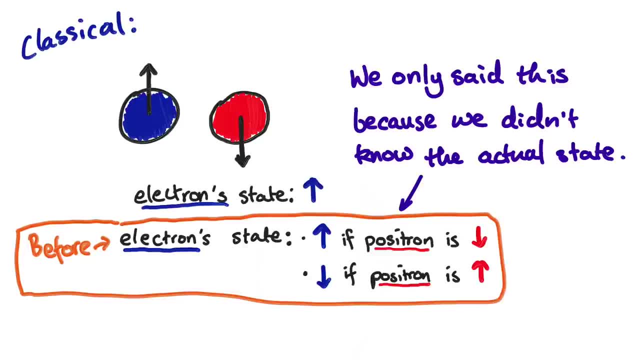 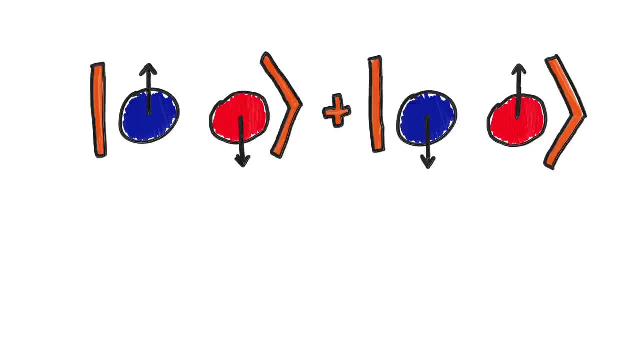 I didn't know which case it is that I had to describe them like this, But in the quantum case there isn't this way out. The particles are apparently doing both of these things, and so there isn't an actual state of the electron that we can. 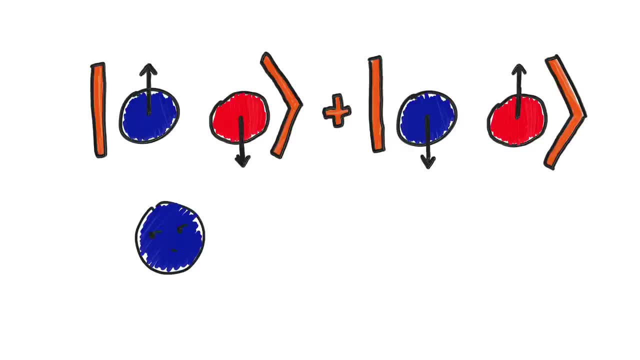 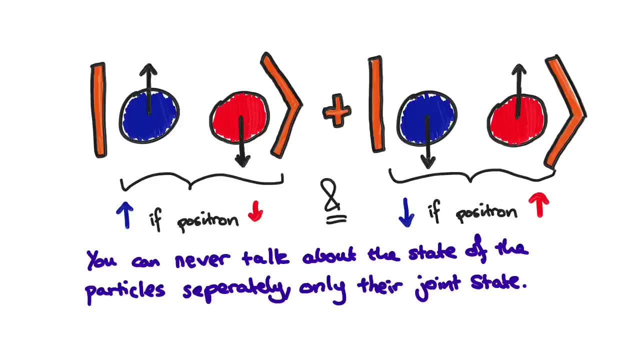 talk about The electron is not actually just up, It's both up. It's up if the other is down and down if the other is up. You can never talk about the state of these particles separately, only their joint state. That's entanglement. 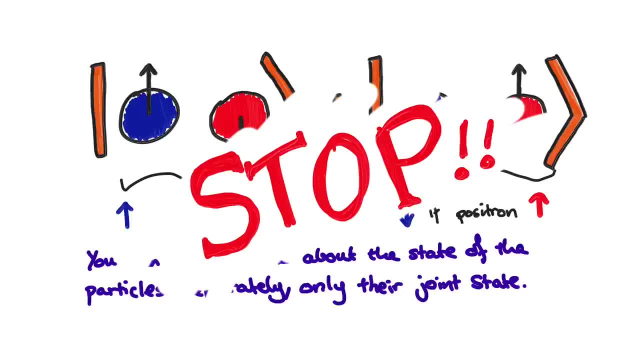 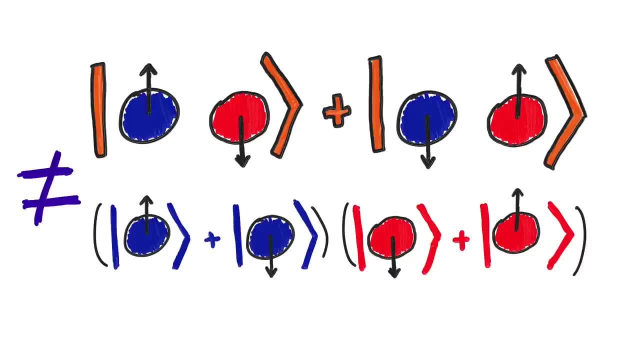 But you might have an objection to this. Can't you say that the electron state is a superposition of up and down? Well, there are two ways to show that this isn't the state of the electron. The first is just mathematically showing that these two states aren't equal, but that's. 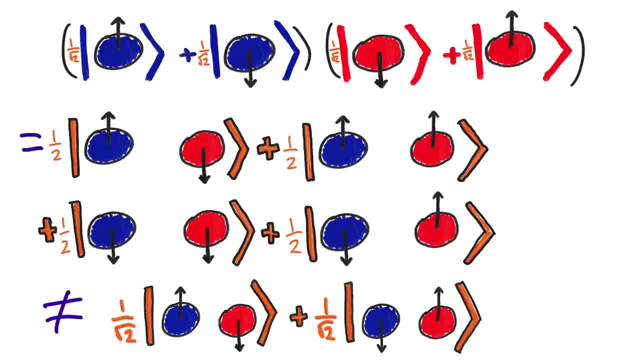 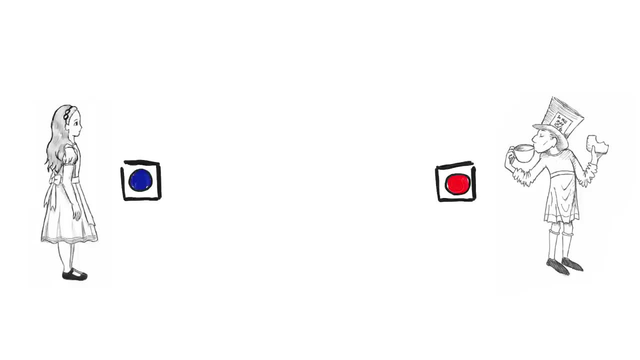 a little bit boring. So instead let's see that this is the state of the electron and see if this would lead to a contradiction. Suppose Alice takes the electron and Bob takes the positron. We'll assume that the state of Alice's particle is a superposition of up and down and the state of Bob's particle 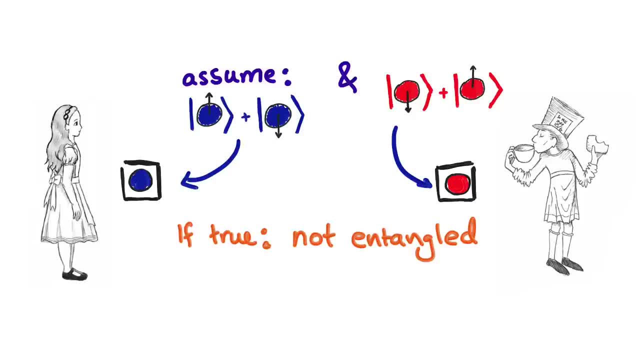 is the same. If this is actually true, then this lets us describe the state of each particle separately, without mentioning the other one. Then say, Alice measures hers and finds it to be up, and so her state collapses, but Bob's doesn't. He can measure his and can still get up as well. This means they start with. 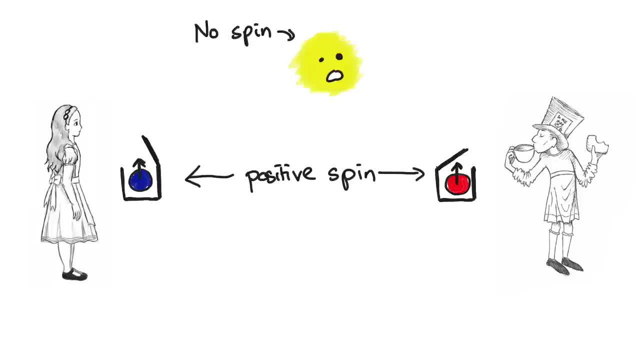 a photon with zero spin and they get two particles with positive spin, which breaks that conservation law. So no, the total state can't be written as these two individual states. The real state is this combination And what really happens is Alice measures hers and say: gets the result up. 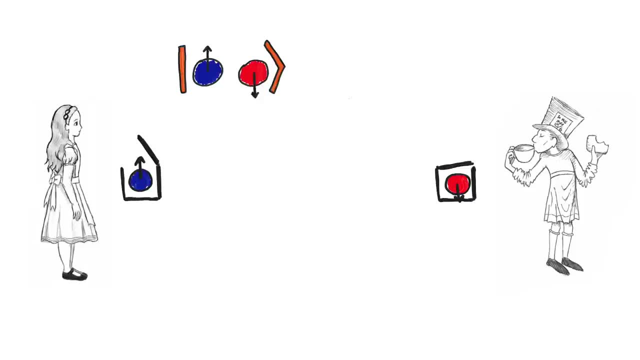 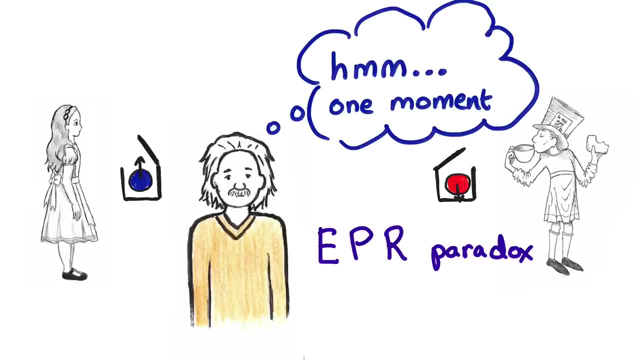 Then that collapses the superposition to just this bit. So now Bob will definitely measure down, and the total spin is still conserved, So we see that we have to believe that the particles are entangled to explain this. It was Einstein, though, who realised the extraordinary consequences. 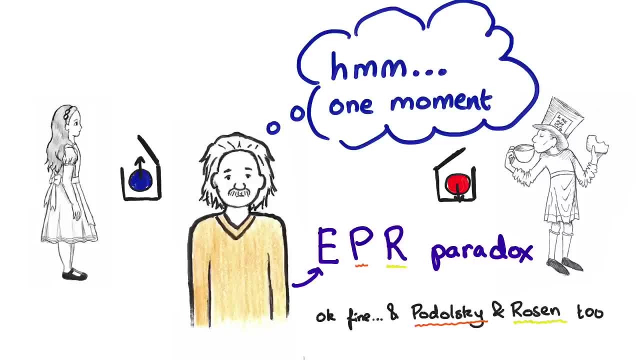 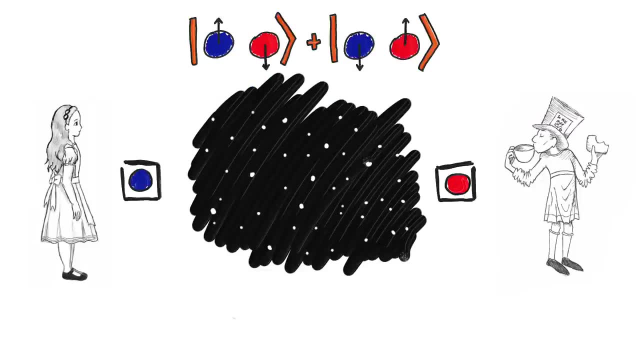 of entanglement. and it's very simple. Let's get Alice and Bob to go very far away from each other and then do the exact same experiment. Notice something: Alice's measurement of her particle affects Bob's particle, because Bob's has to be the opposite. 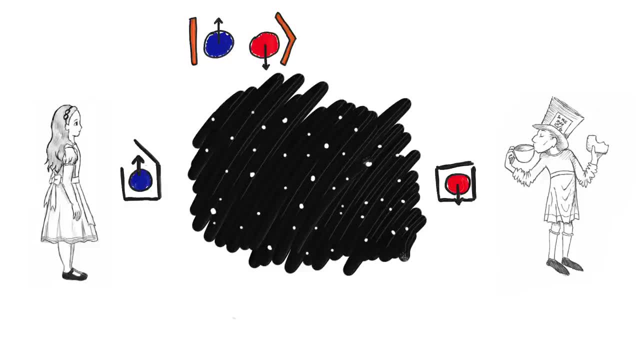 But even worse, that effect has to be instant, because if Bob measures his particle a split second after Alice, he needs to still get the opposite result. So there can't be any delay in how quickly Alice's measurement affects Bob's. Somehow the message from Alice's electron to the positron 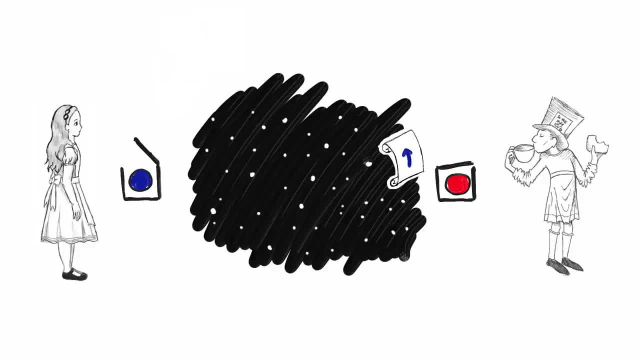 travelled instantly. In other words, this effect is non-local. The issue is that this seems to contradict Einstein's theory of relativity. In that theory, no information can travel faster than light, And the reason is that if it could, then you could cause things like time travel and the grandfather paradox. Einstein thought that this would be enough to convince people that quantum theory is silly, But what really happened was the scientific community of the time weren't able to come up with a good answer to it, and instead just decided to ignore it. It wasn't until much later that people cared, and even later that it was proved that the sort of spooky action at a distance in quantum mechanics